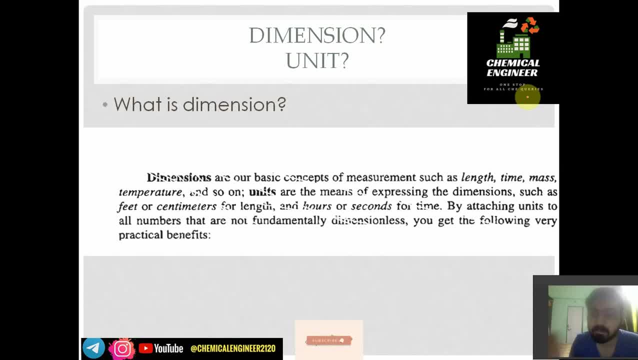 you should have clear understanding. okay, dimension and unit, what is difference between them? so dimension are our basic concept of measurements. so measurement means length, time, mass temperature, luminous intensity, etc. so all these things that we can measure like length, time, mass, temperature, they are known as dimensions. dimensions. you know, you have studied in 10th or 12th that m, 0, l, 1, t, 1, like, suppose. 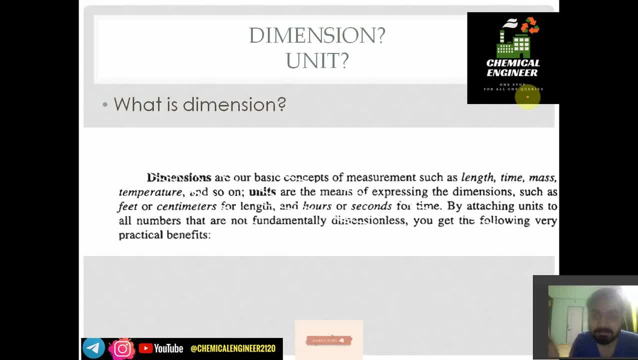 l, 1, t minus 1 is for velocity, so l, t, T, M, those quantities are the dimensions, okay, and units. so in order to describe dimension we use units. so units are nothing but to describe dimension in certain thing, like suppose, we say, suppose two person are talking, one says that, uh, time is two, okay, so two, so two holds. 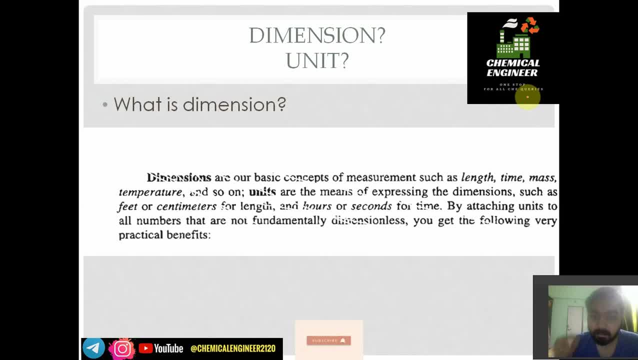 nothing, no meaning, but two hour, two second, two minute. this thing will hold some meaning, okay. so that is why we use units, so that is why we have developed units for everything. every dimension has unit, okay. so this is a basic difference between dimension and units. so dimension is a quantity. 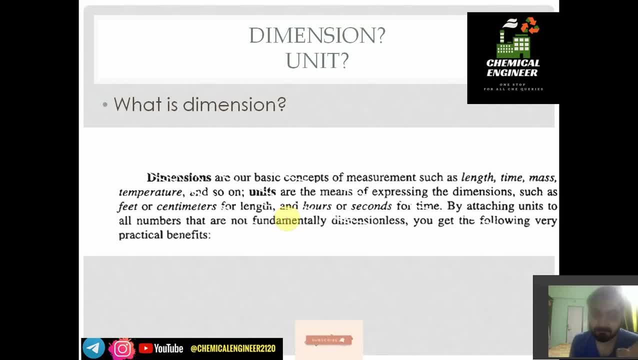 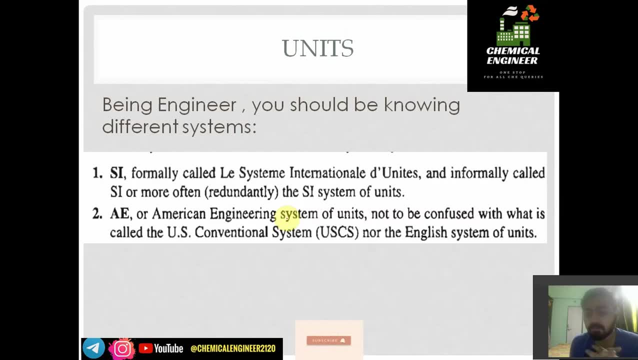 and unit is its expression, expression of dimension, okay, so you should have clear understanding about it. so, being engineer, you should know different unit systems. so first unit system that we all use is SI, also known as lay system, a international d units or units. so SI is the system, international unit. that is what we all are going to follow. so units. 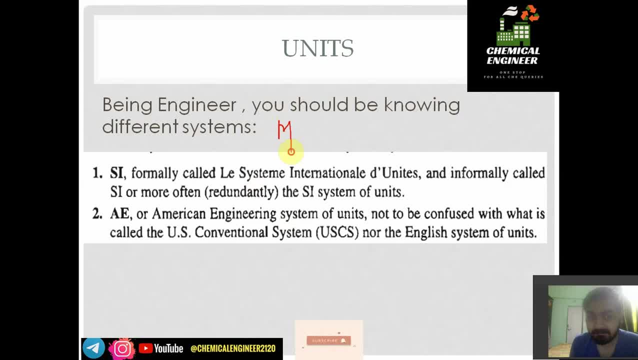 of labour and labor of labour, he assistance sector for every unit and therefore iföt quantity c 240 and ift such so podcast like for the factory aesthetics, current and modern and differently, you know, related to this one. so you will understand now the purposes of this. 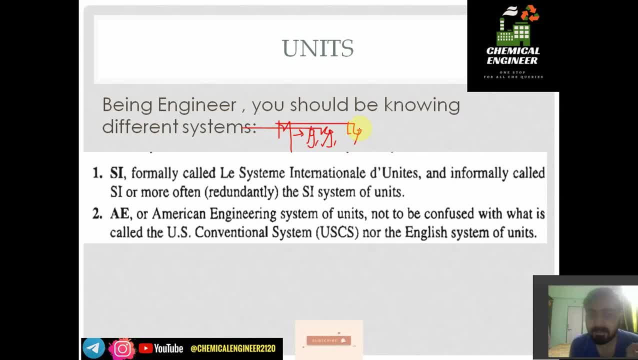 weight is pound, so different units are derived and interrelations are present between them. okay, so you should know the names of the systems. so first is si, second is fps, that is foot pound. second, then you should have a cgs system, centimeter gram second system. then then comes 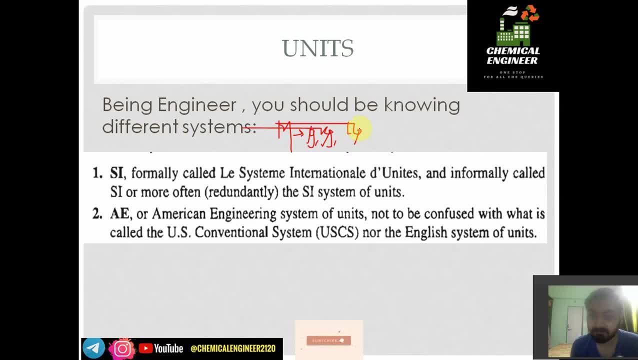 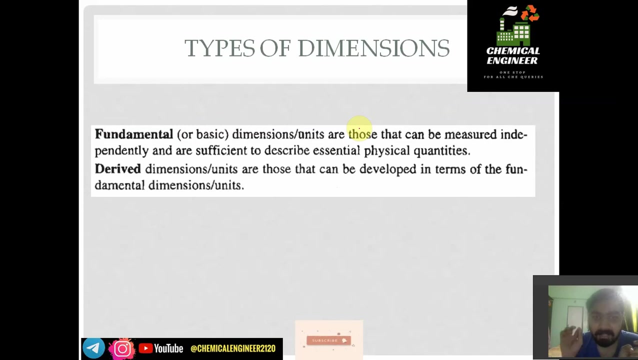 the si system. then comes the american engineering system. so american engineering system is nothing. that is also the fps, okay. so you should have known that the systems are different and they use different units, okay. so what are dimensions? we have discussed length. mass time are the dimension. now, there are two types of dimensions, so fundamental and derived, okay. 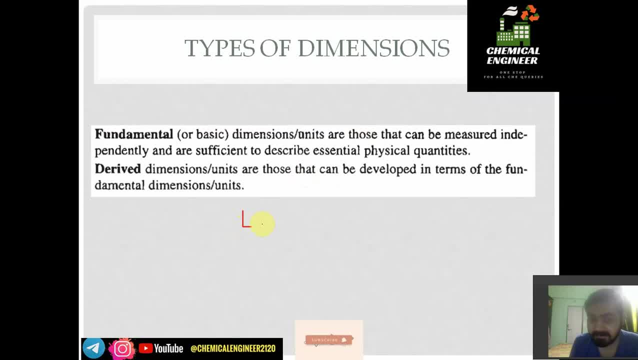 now suppose we have length as one dimension and time as other dimension. okay, length and time as two dimensions. so these are independent dimension or we can say fundamental dimension. fundamental means they cannot be break into smaller sections, so length and time are the fundamental. but from length and time we can make velocity, so velocity is given as length. 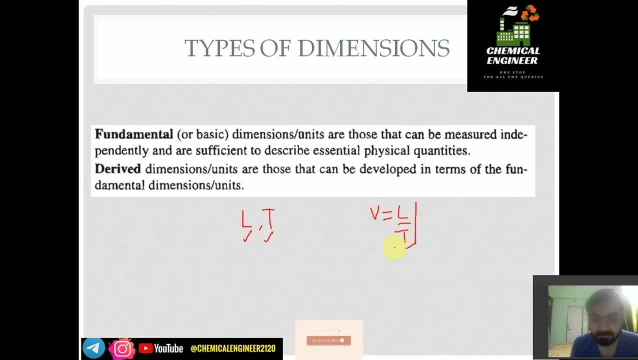 divided by time. okay, so this dimension of velocity is will become a derived dimension or derived unit, like length as a unit of meter, time as of second, and velocity will have unit of meter per second. so it is derived from length and time. so these two are the different types. 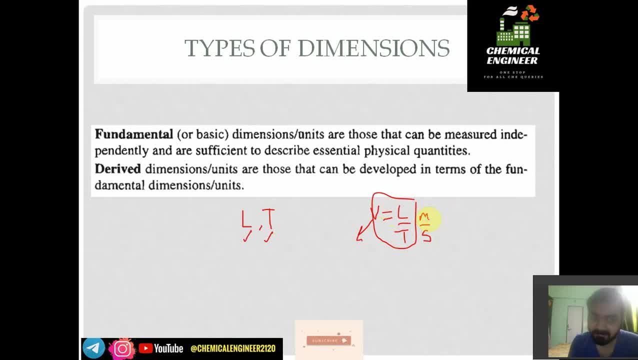 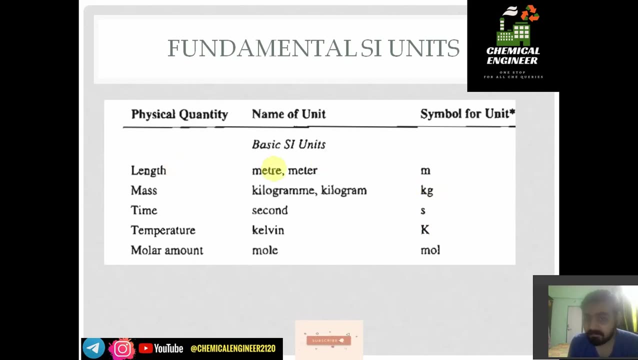 of dimensions, length and time are the fundamental, while velocity, force are all the derived- okay, dimension or derived units. so in sl unit we use length in unit of meter mass, in unit of kilogram, time, in unit of second kelvin, in unit of k, that is, kelvin or temperature. 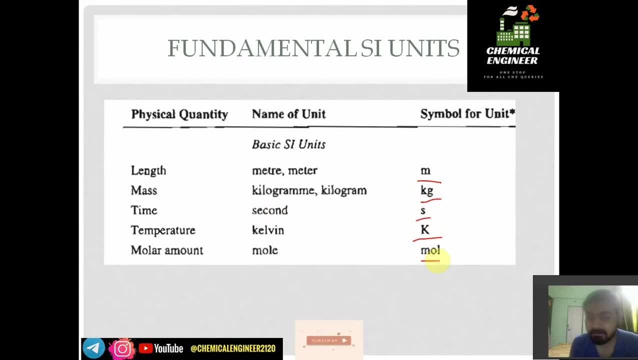 is in the unit of kelvin and molar amount is in the mole. so in sl unit we have seven quantities as a basic quantities. here i have only discussed five quantities. so qurition 1 of this video is you have to find other two of those upto 3 quantities. 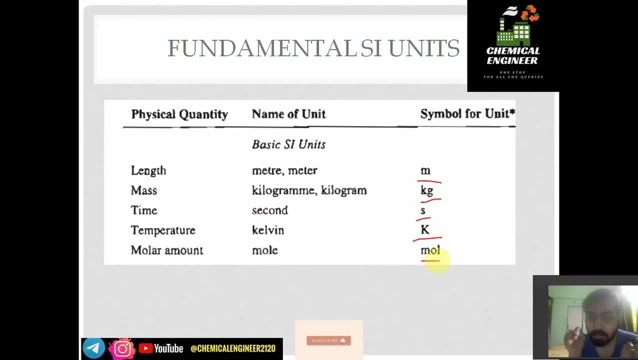 which we have forgotten to add here. you have to just name them, okay, and their unit. so please, if you are watching this video carefully, please comment. okay, so these are the five quantities. we have two others you have to find and give me the answer, which are the seven basic quantities. 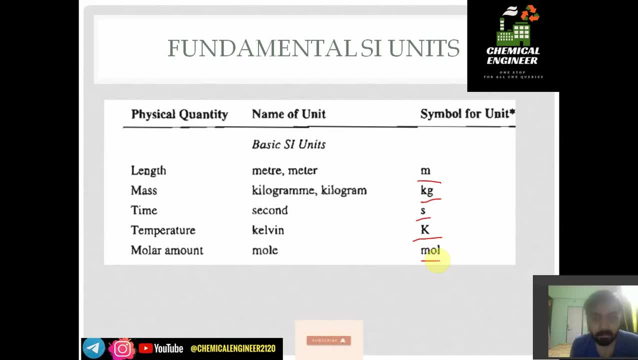 that is selected by sl unit. So, friends, last question: I would like to ask for answers, to make the question a bit further. and look here there is something to write here. K is not capital, so every time you have to write kg in like this, only like K: small meter M is always small, second s is always small Kelvin. 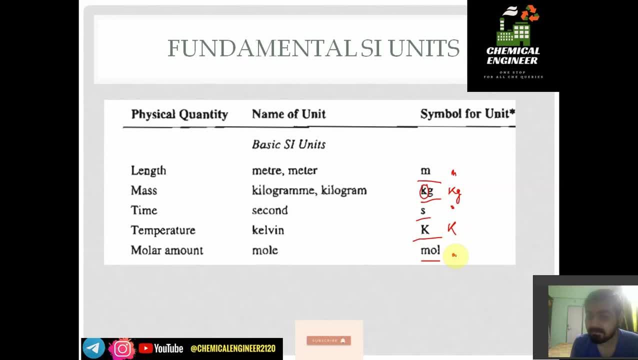 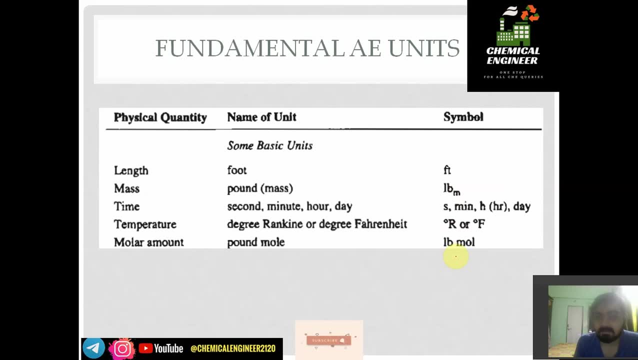 K is always capital in mole mo, L is in a sentence or in a lowercase, okay. similarly, in that American system we measure length in terms of foot, mass in terms of pound. and, yes, foot is given as F, T, pound of mass is given as L, B, M in a small then time in. 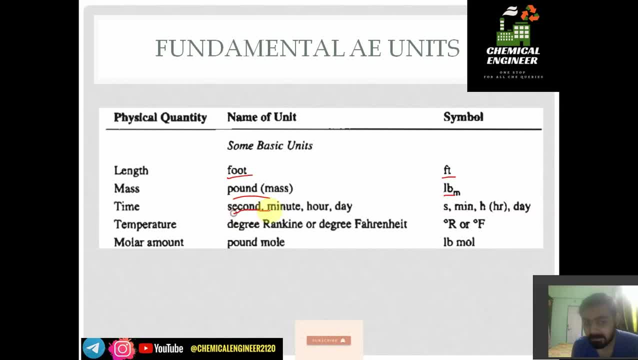 FPS system or American system. they may use different quantities like second minute, our day s min HR or day okay. so you should have clear understanding. in temperature we have degree Fahrenheit and degree Rankine in a unit. in that unit we have Kelvin and molar amount is calculated. 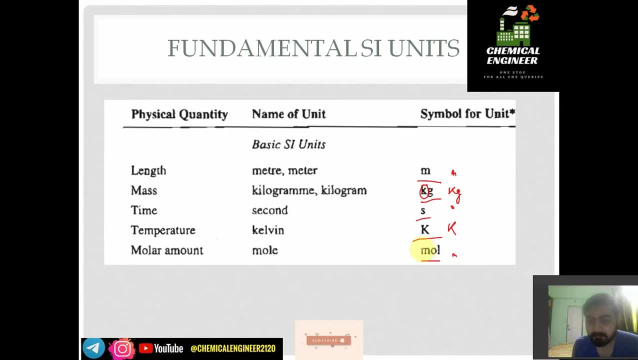 as pound mole or LB mode. here it is also known as gram mole. okay, so no need to get confused. this also. this is also mole. is simple mole? return anytime you will see that simple mole is written. it is gram mole, okay, if it is not specified pound mole or something like that. it. 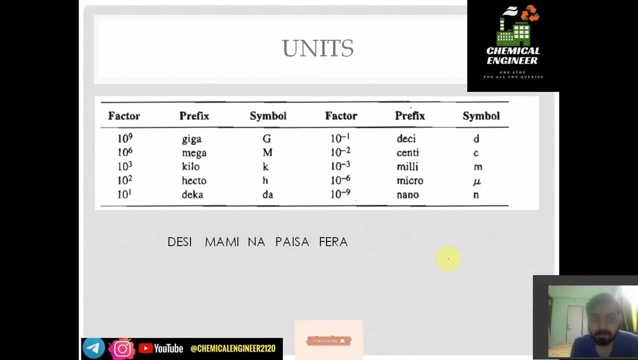 is gram mole, always okay. so units, now we have seen the units. now we have different. uh, I would say we have the dose of moles. now we can write down that is the weight multiplied by the weight of the cold water temperature. so the total temperature of the javelin is 1 chamber in the unit. so 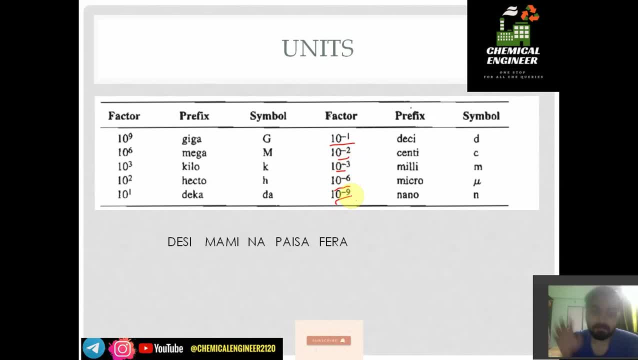 that it is 3phi. that means the temperature of the Javelin is 2.3 degrees, and so on. okay, so let's go with a minus 1 and the difference between the two equations is that the temperature of the loaded magazine is 10 degrees to minus 3, so that is exactly 2.0 into 10 degrees and you can write: 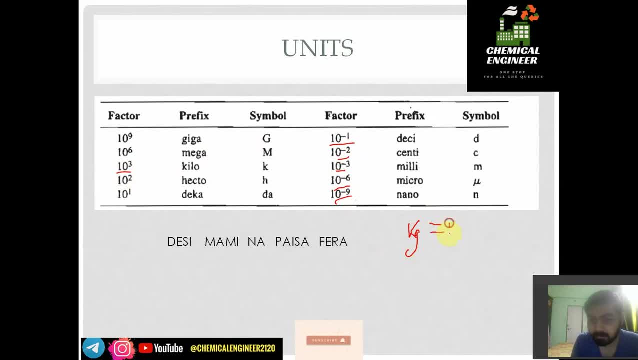 to 3, so that we can write as 10 raised to 3, that is, in terms of k, we can write 10 raised to 3 gram. okay, okay, so that is, you should have knowledge about this in your plus 2, or that, so always, 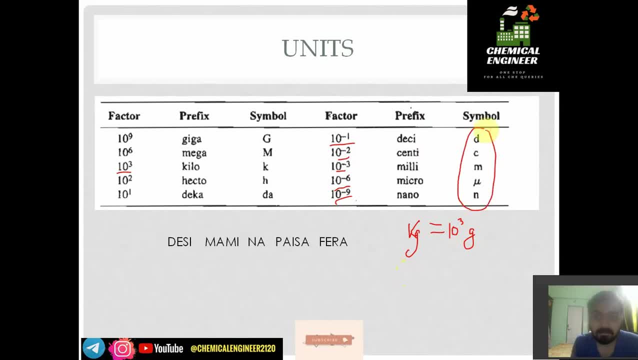 remember that those quantities which are going to the 0 point, something it is always written in terms of smaller or lower case, like desi, is given as d, e, c, i. so d, small, d, centi is c, milli is m, micro, is mu, nano is n, small, n, and all the quantities which are bigger than one. 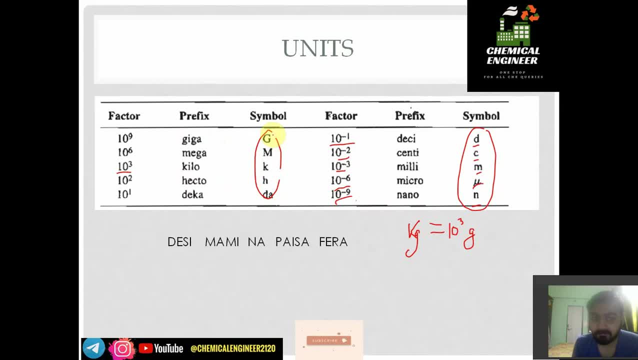 are given as a bigger case or upper case. so we have deca, hecta, kilo, mega, giga, okay. so then we have 10 raised to my mine, okay. so here we have d, e, c, m, i, m, i, n, a. so 10 raised to minus 9 is 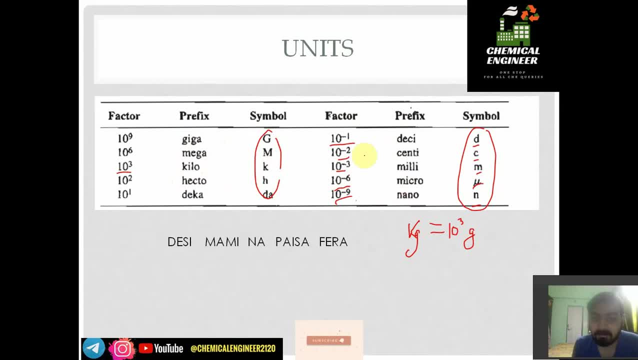 nano, then we have pecto, then we have farah. so the difference is 10 raised to 3 difference okay. so difference between the two is 10 raised to 3.. similarly, in this case, this is kilo, mega, giga and farah, 10 raised to 15.. 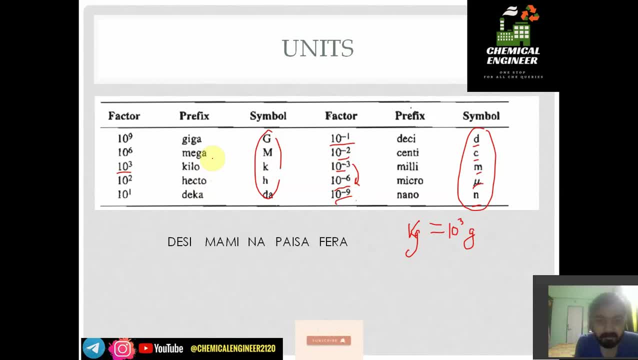 and tata is 10 raised to 12.. so this is how we can remember them. so this is for gujarati people's desi mami na paisa faira, to remember the this: desi mami na paisa faira, so you can remember it. 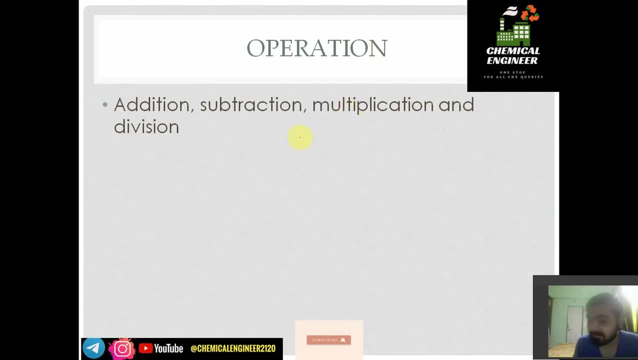 and operations. okay, so we have discussed different units like mass is kg, length is meter. what is this? length is meter, time is second. now different operation. we can try. so let us do operation of addition: addition. so we cannot add two different quantities, like we cannot add one kg. 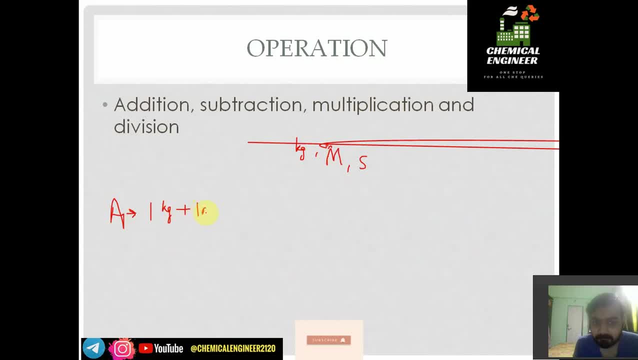 plus one meter. okay, so this will be wrong. we cannot add different quantities or different units. we can add two similar unit like 1 kg plus 7 kg, so it will yield 8 kg. okay, so this unit gives 8 kg. so we can add only two units having same units. okay, so same dimension it should have. we can add: 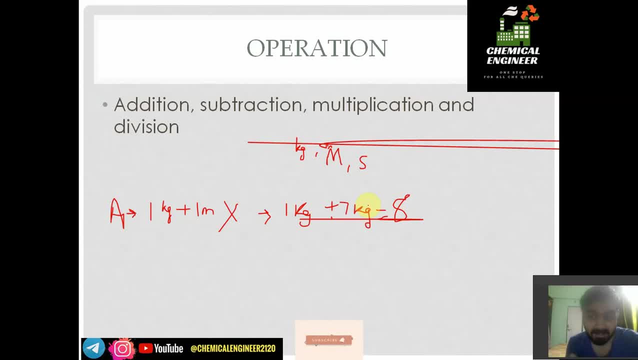 as well as we can subtract only when they both have same dimensions. okay, we cannot do like this: 1 kg plus 1 meter or 1 kg plus 1, second, 1 kg minus 1 meter, like that. we cannot do that in multiplication, suppose two units are there. that is force equal to, given as M into a, so dimensions. 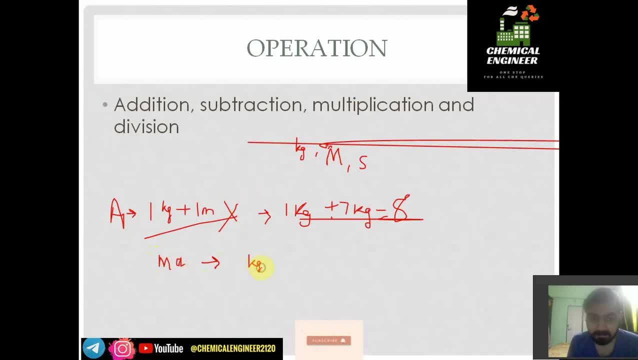 of mass are kg and dimensions of acceleration are meter per second square. so when we want to multiply and divide, we directly do its multiplication and division of units like force equal to ma, so a is prepared from mass by second, that is velocity divided by second. so meter per second square is the unit of acceleration. so we can directly. 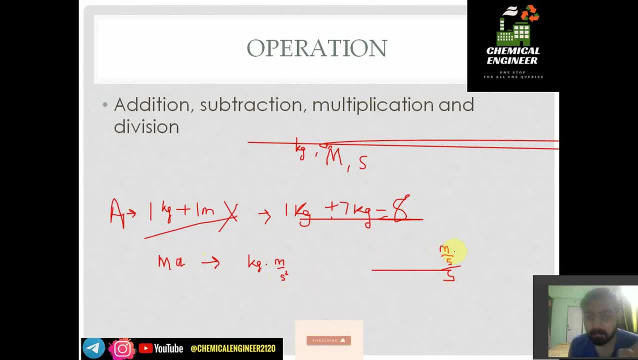 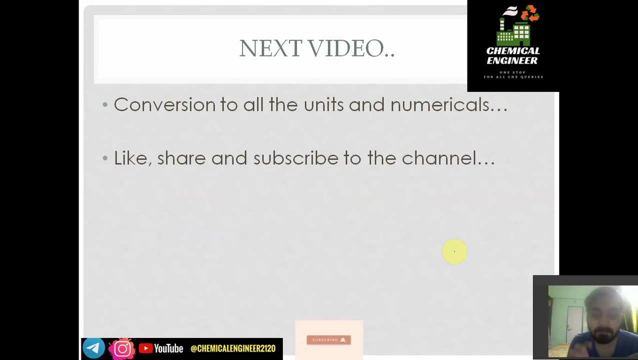 multiply and divide it. but we cannot add and subtract to the different units. but different units can be multiplied and divided. so this is a basic we have covered. in next video we will see about our different units and their conversion, inter conversion, like how to convert kg to pound, Kelvin to Rankine, Kelvin to 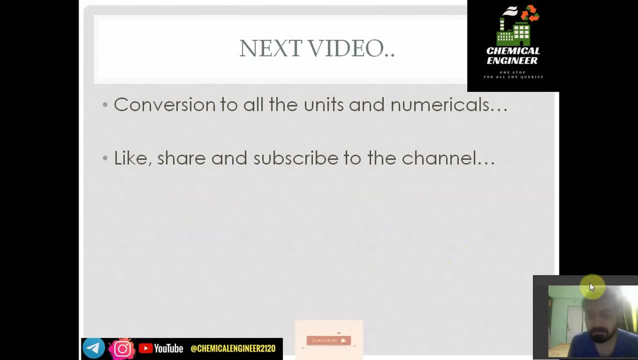 Celsius and all. so thank you for watching this video. we will meet in next video. okay, so thank you for watching. subscribe us. subscribe us.